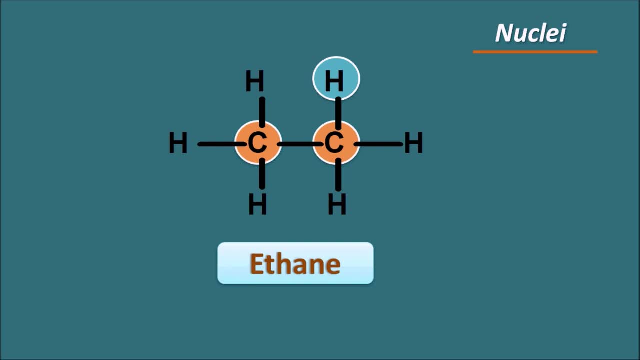 again, here all the hydrons are equivalent because they are similarly attached. So ethane is having the two carbons and six hydrogens. These hydrogens can also be called as protons. So it is having the two carbons and six protons, but interestingly here the carbon cannot give. 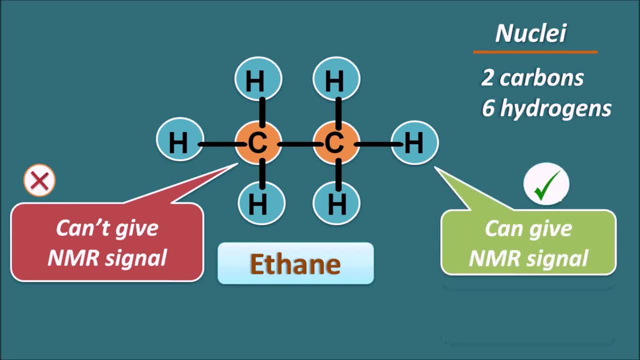 the another carbon of match than음�arioства. So it presents the cono mahdollius electron locus astwo's Отастて, 그다음에ankaghetti온, бесп, Germany, beh館을 보eeeee. NMR signal. On the other hand, here the proton can give the NMR signal. So within the ethane, 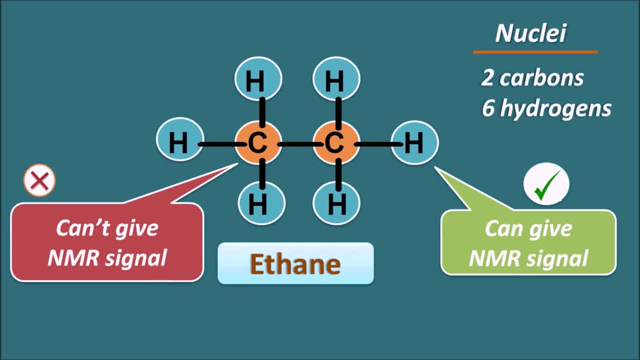 molecule. two types of nuclei are there. one is a carbon and another is a proton. but proton can only give the NMR signal. The reason is the carbon, which is the 6C12, is having the spin- quantum number i is equal to 0, whereas the proton, which is 1H1, is having the spin. 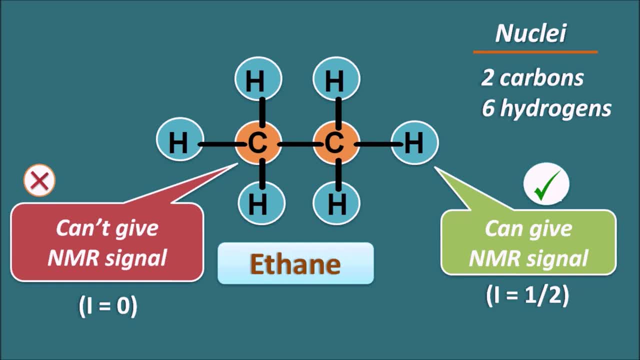 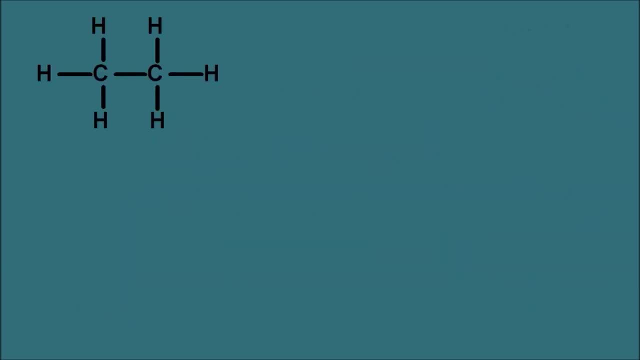 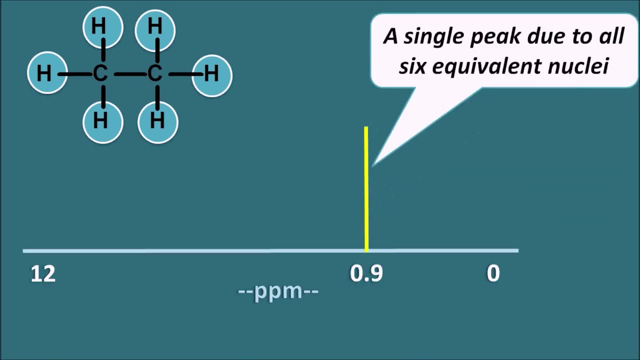 quantum number i is equal to half. So in the NMR the nuclei with i is equal to half can only give the NMR signal. So now, if you take the ethane, ethane is having the six equivalent protons. since all the protons are equivalent, they will give a single. 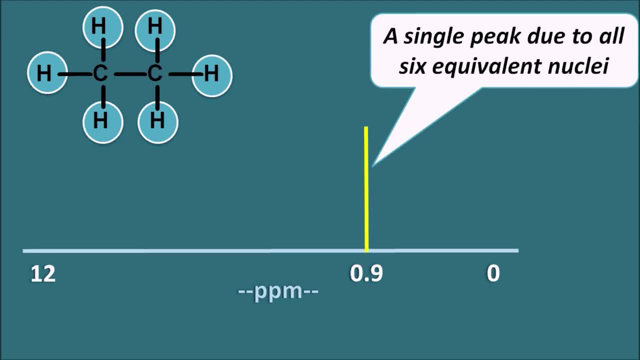 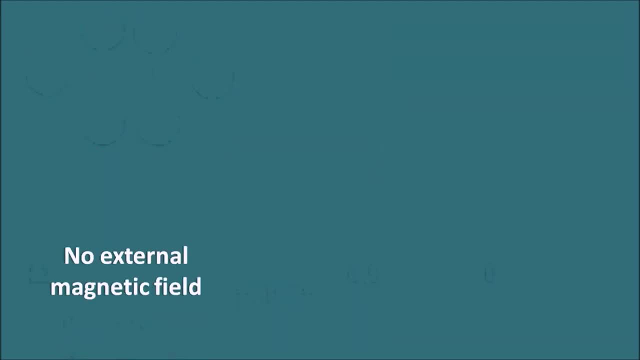 peak in the NMR spectroscopy. but here the proton can give the NMR signal when we apply the magnetic field externally. So when there is no external magnetic field field the nuclei will not have any spin. so the spin is zero. but when we apply a magnetic field, 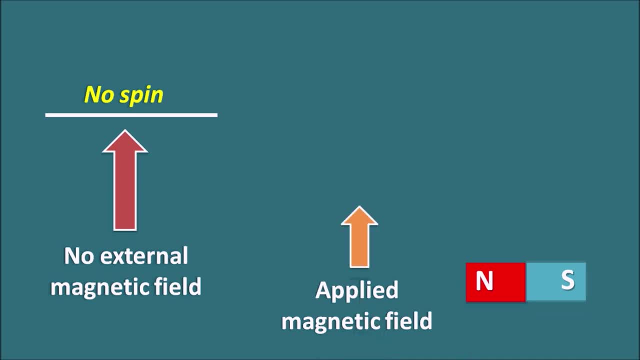 under the influence of this externally applied magnetic field, the nuclei can have the two spin states. The spin state with the low energy can be considered as a ground state and another spin state with the higher energy can be considered as a excited state. So, under the applied magnetic 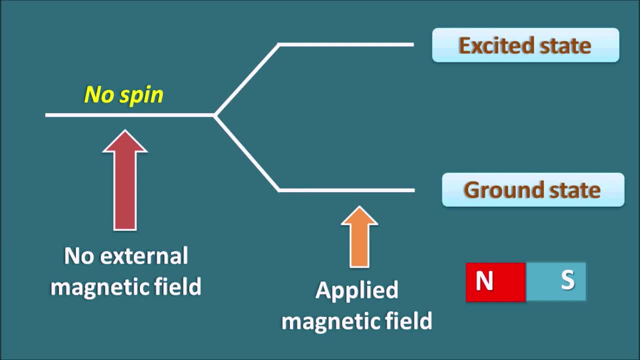 field nuclei can exist in the either ground state or in the excited state, and when we supply the energy in the form of electromagnetic radiation, this electromagnetic radiation will promote the nuclei from the ground state to the excited state, which is observed as a signal in the NMR. 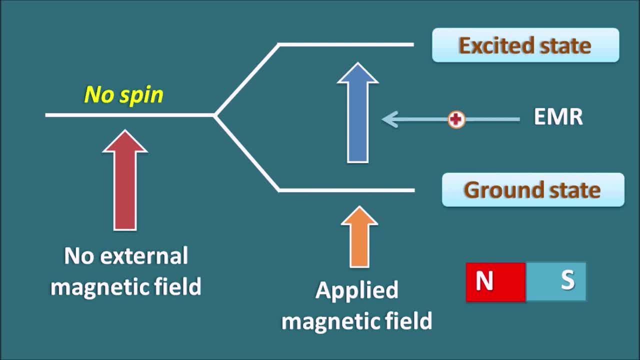 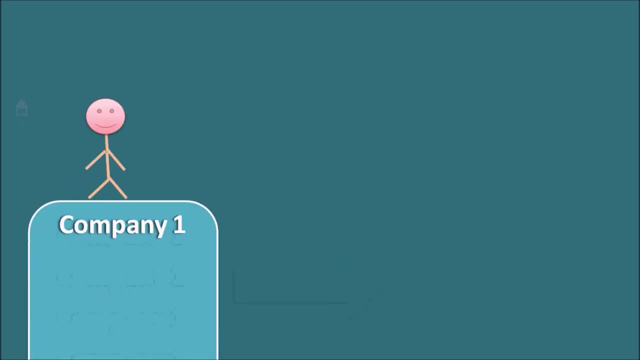 spectroscopy. So NMR spectroscopy is a simply one type of absorption spectroscopy observed by the nuclei having spin quantum number i is equal to half. This situation can be simply illustrated by a common example. Suppose a person is working in a company one and until. 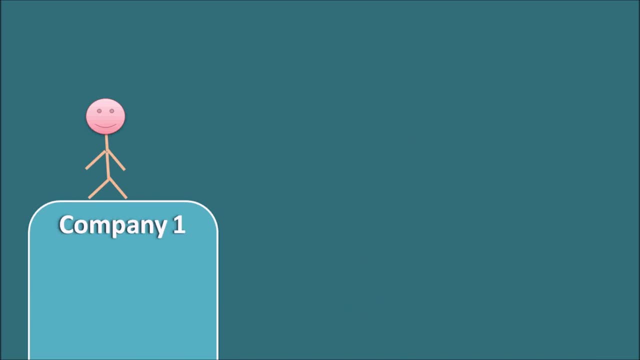 unless there is no new offers. the person goes on working in the company one and at one time, suppose a new company is going to be established which is a big company compared to the company one, and they have given an offer to the person. Now the person can jump to the company two In order to shift of the 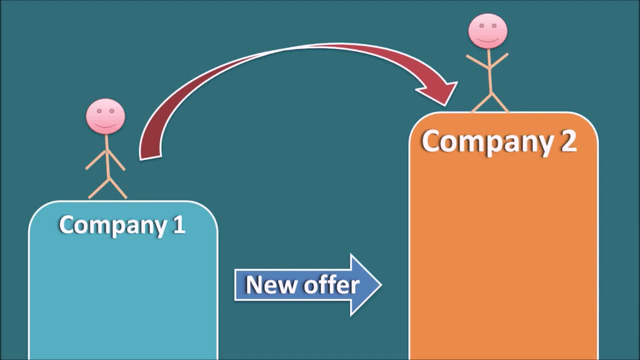 person from the company one to the company two, there should be some advantage. Suppose either salary is increased or designation is increased. there is a chance of shifting of the person from the first company to the second company. So now that we can compare the situation to the NMR spectroscopy, The new offer offered by the big 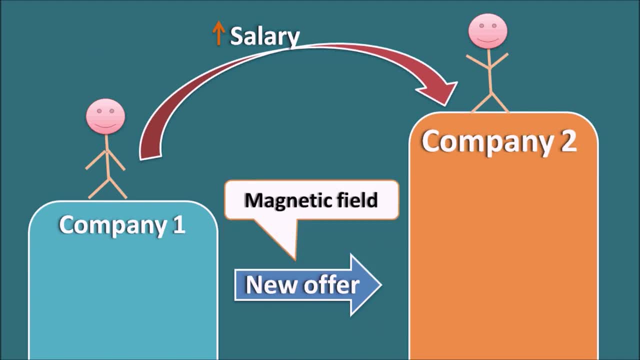 company is nothing but the magnetic field we are applying, and hike in the salary is nothing but the energy we are giving the form of electromagnetic radiation. So when we apply the magnetic field, the nuclei will have the two chances like ground state and exit state, but it can jump from the 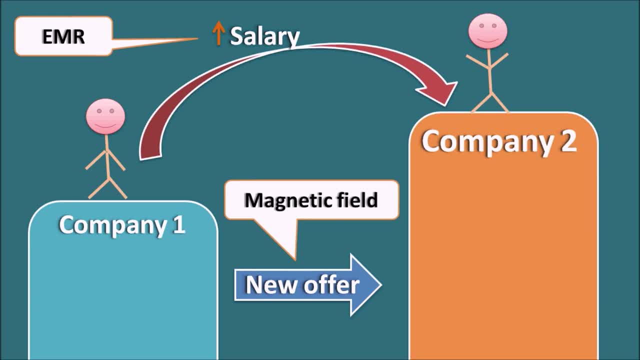 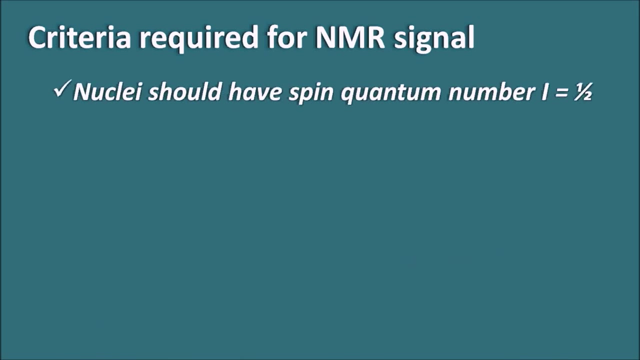 ground state to the exit state when we supply the sufficient electromagnetic radiation which resonates with the energy gap between the two states. So that is the NMR nuclear magnetic resonance. Now what are the criteria required for the NMR signal? Just, we have seen that nuclei should have a spin quantum number i is equal to 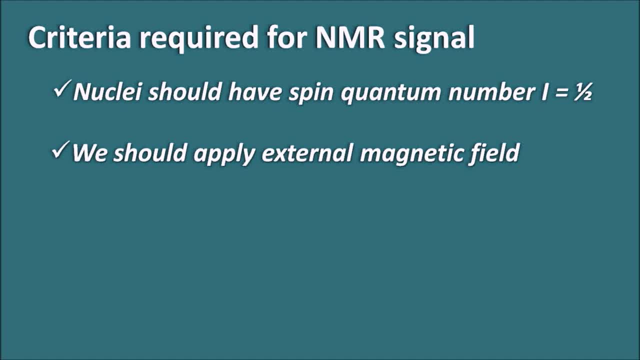 half and we should apply external magnetic field and under this influence only the nuclei can have the two spin states. and then we have to supply the sufficient energy in the form of electromagnetic radiation. that resonates with the energy gap. For most of the nucleus, the energy gap resonates with 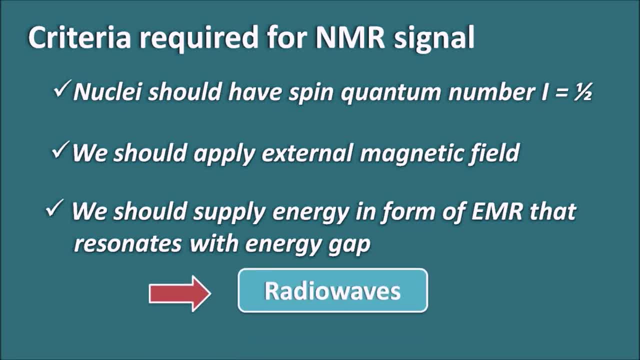 the radio waves. so we can supply the radio waves as the electromagnetic radiation in order to observe the NMR signal. But here we can have a doubt that why the spin quantum number of the nuclei should be equal to half in order to show the NMR signal. Now let us see what is the reason for a nuclei to have. 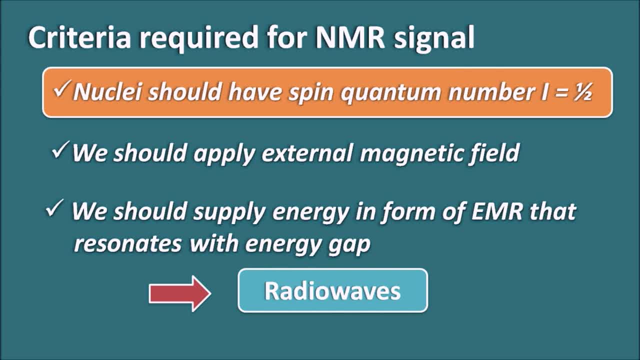 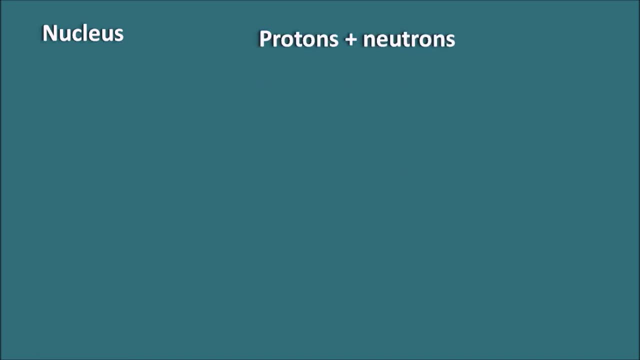 i is equal to half in order to show the NMR signal. Before going to discuss why i should be half, let us, which have the I is equal to half and can give the NMR signal. So nucleus is composed of the two important components, protons and neutrons, The spin quantum. 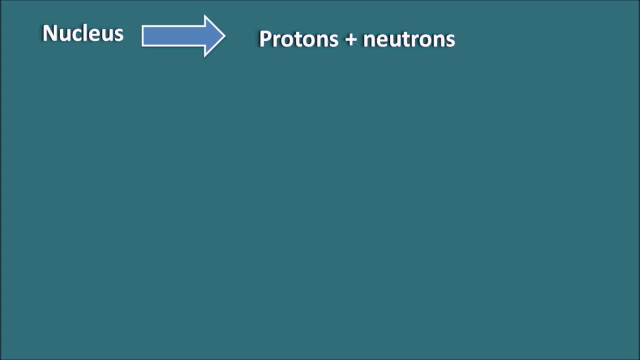 number I value is with maybe either integer or non integer, and it may have the any values like the 0, half 1, 3 by 2 and so on. Even we cannot assign the I value just by seeing the particular atom, still we can have a logic in order to. 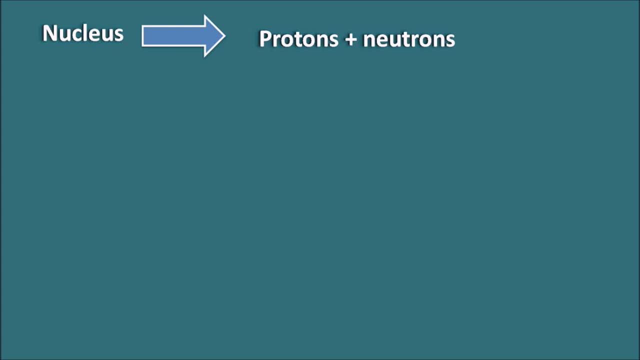 remember which type of nucleic can have the. I value as half as zero as one. Suppose an atom is having the even number of protons and even number of neutrons, then I value will be 0.. So examples include the 6c12 already we. 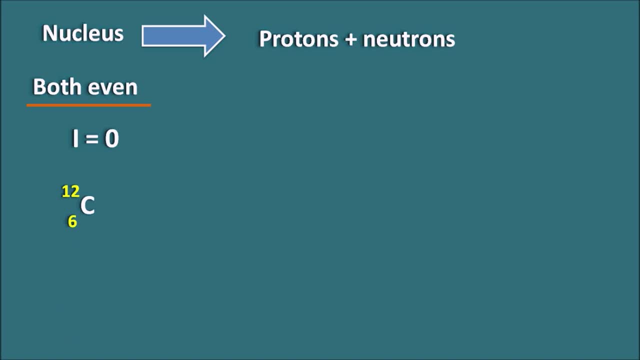 have seen that carbon cannot give the NMR signal because the I value is 0. Now the carbon is having the 6 protons and 6 neutrons. because the number of protons and number of neutrons are even, it will have the I value as 0 and it cannot give the NMR signal. Similarly, another 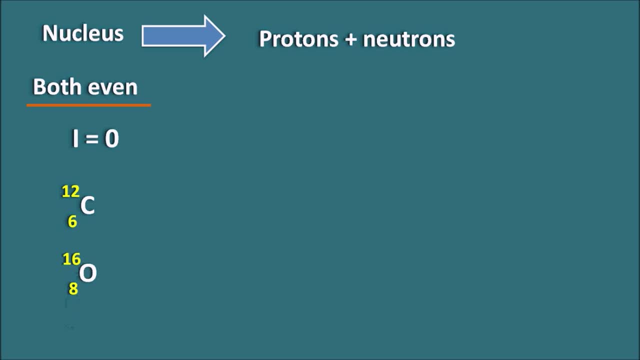 example is the 8O16, the oxygen, again having the 8 number of protons and 8 number of neutrons. both are being even and similarly the nuclei which are having both number of protons and number of neutrons as odd will have the I value equal to 1.. Again, the examples include 7 and 14. 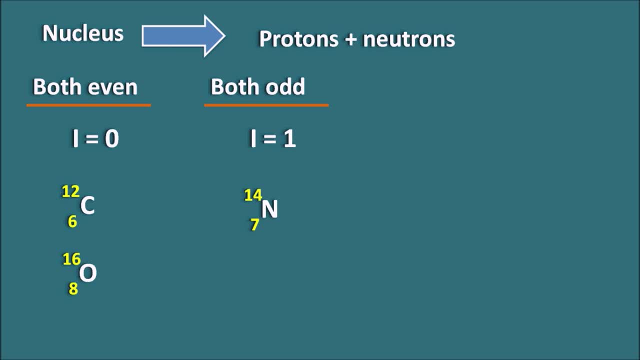 so nitrogen. nitrogen is having the 7 number of protons and 7 number of neutrons. being both are odd, the I value will be equal to 1.. Now if a nucleus having one of the component as odd and another component as even, for example, it is having the odd number of protons and even number, 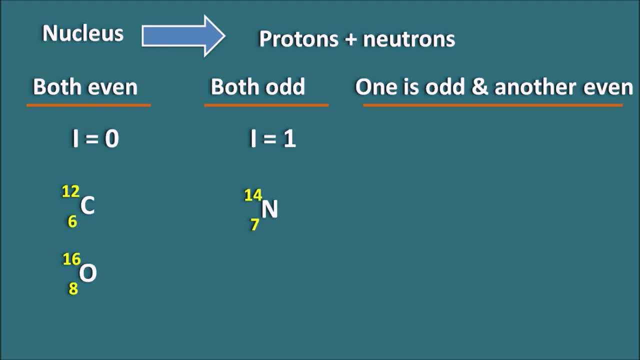 of neutrons, or even number of protons and odd number of neutrons. then I value will be either 1 by 2, 3 by 2, 5 by 2, and so on. So here all the neutrons will be equal to 1.. 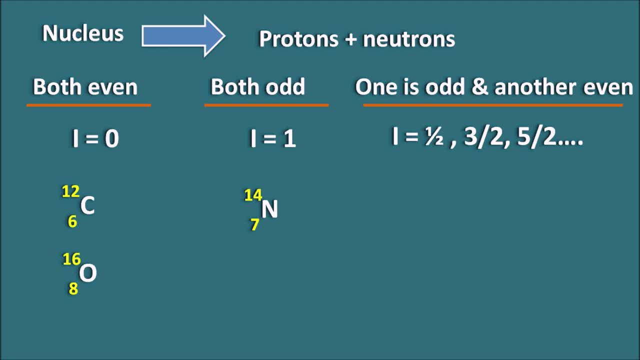 All such type of nuclei cannot give the NMR signal, because we have seen that for a nuclei to show NMR signal I should be equal to half. So among these nuclei, we can remember those nuclei which are having I is equal to half so that they can give the NMR signal. 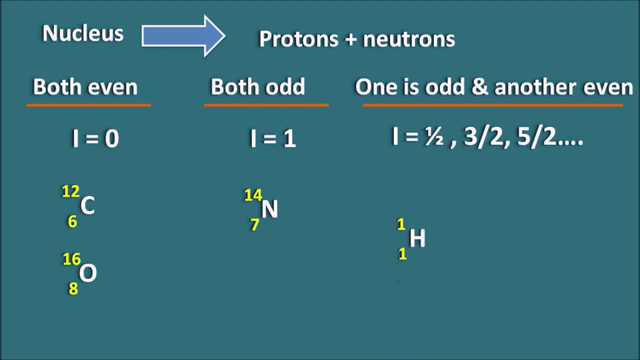 Now the nuclei which are having- I is equal to half- include 1H1. simply we call the proton, So 1H1 is having 1 proton and 0 neutrons. Similarly, 6C13- isotope of the carbon- 6C13. 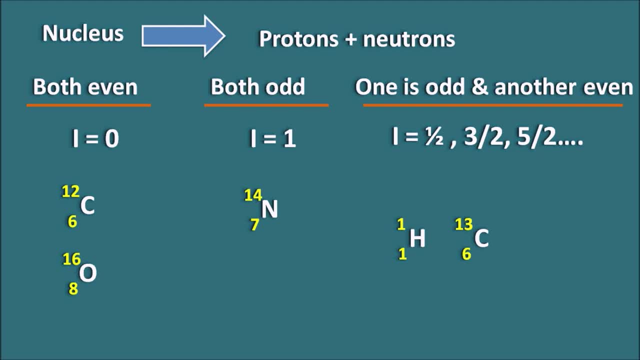 is having 6 protons and 7 neutrons. That means it is having the even number of protons and odd number of neutrons And another nucleus, the 9F19.. So fluorine is having the 9 number of protons and. 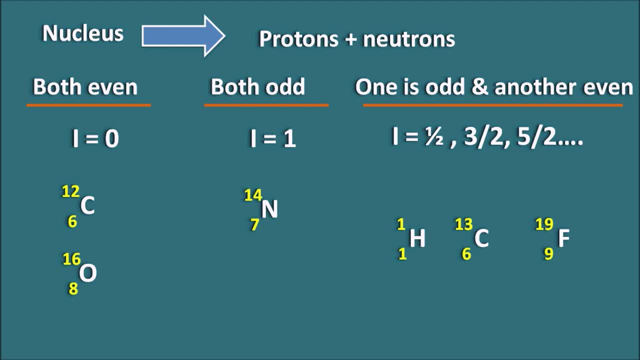 10 number of neutrons. So it is having the odd number of protons and even number of neutrons. Similarly, 15P31: it is also having the 15 number of protons and 16 number of neutrons. So these are the examples of the nuclei which are having either odd number of protons and even. 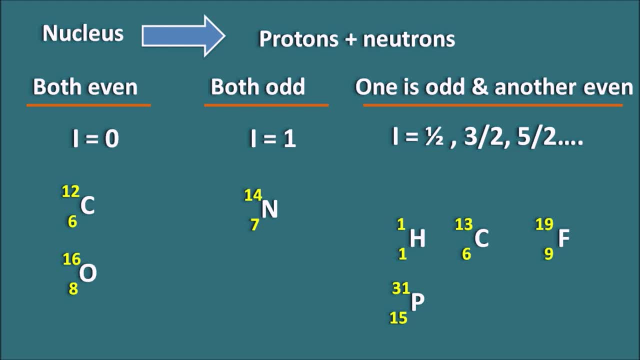 number of neutrons, or even number of protons and odd number of neutrons. So these nuclei can have the I is equal to half and these nuclei can only give the NMR signal. Here we should not confuse that every nuclei with 1 is odd and n is even will have the I is equal to half. Because when 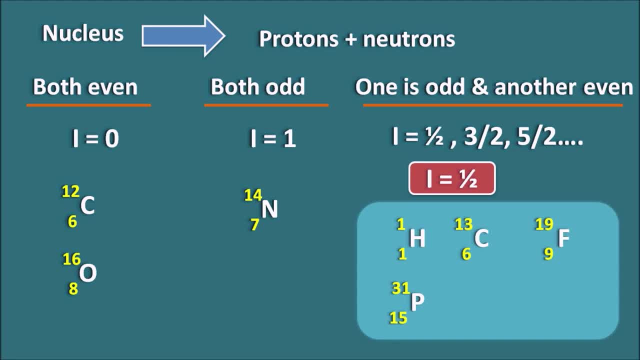 1 is odd and n is even. they may have. I value as either half, 3 by 2,, 5 by 2 and so on, And among these, only these nuclei can only have the I is equal to half and can give the NMR signal. So 1H1 we call the proton NMR and 6C13 we call the 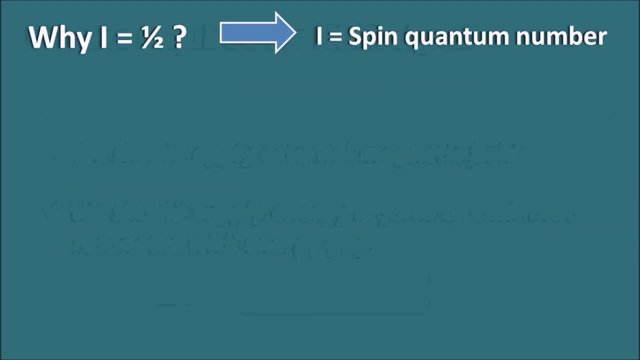 carbon NMR spectroscopy. I is nothing but the spin quantum number. In order to see why I should be half, we can define another parameter: magnetic moment number. The magnetic moment number indicates the number of the spin states of the nucleus. So the number of the spin states of the nucleus is 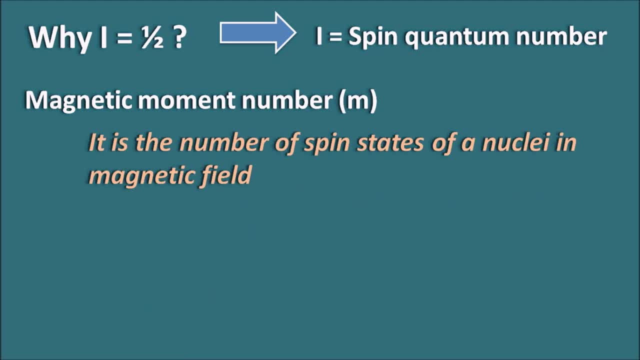 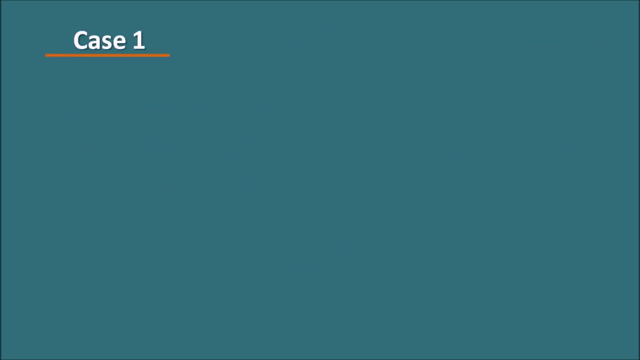 the number of the nucleus in the externally applied magnetic field, Where m is given as 2 into i plus 1, where i is the spin quantum number. Now let us take a case 1, where i is equal to 0. When i is equal to 0, what will be the m value, The magnetic moment number? So m is equal to 2 into i plus 1.. 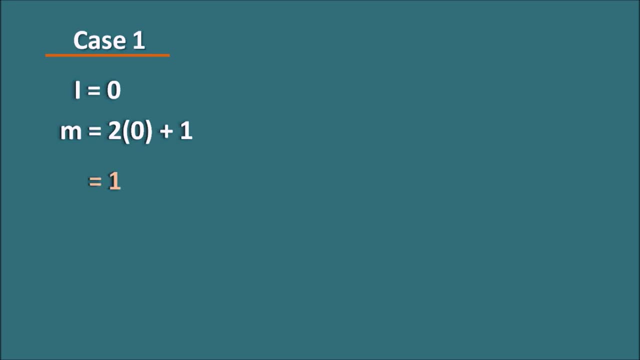 That is nothing but 2 into 0 plus 1.. So which gives 1.. So when i is equal to 0, m is equal to 1.. That means the nuclei will have only one state, And this state of the nuclei will have a spin quantum number as zero. 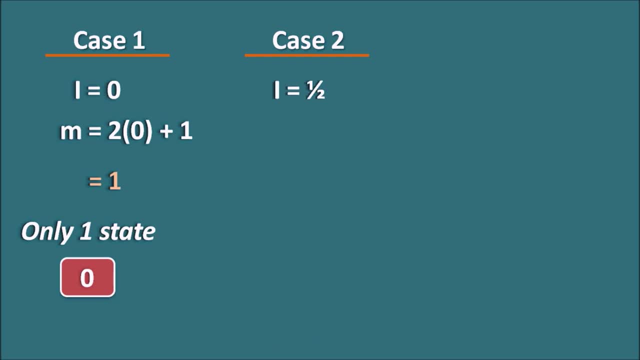 And let us take case two, where i is equal to half and then m is equal to two, into half plus one, so it gives two. So now the nuclei under the applied magnetic field, it can have the two spin states and each spin state will have a spin quantum with minus half as well as plus half. 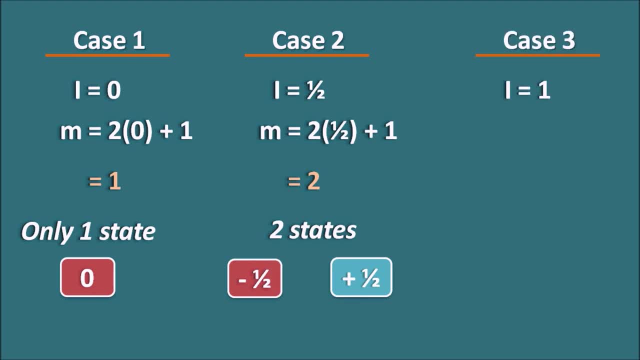 Now let us take the case three, where i is equal to one. So when i is equal to one, m is equal to two. into one plus one that is equal to three. Now the nuclei can have three spin states under the applied magnetic field. 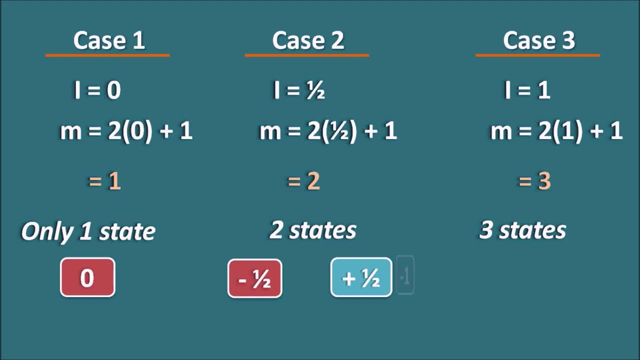 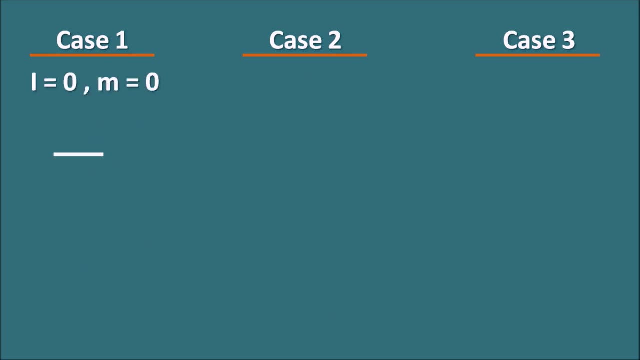 These spin states can have a spin quantum numbers as minus one, zero and plus one. Now let us see why i should be half in order to show the NMR signal. Now let us see the case one, case two, case three. In the case one, we have seen that i is equal to zero and m is equal to zero. 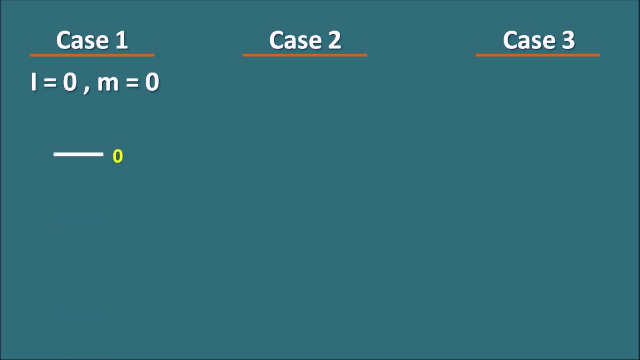 Therefore it will have only one spin state And the spin of the spin state is zero And in the case two, i is equal to half and m is equal to two. So now it will have the two spin states, and one of the spin state is of the plus half. 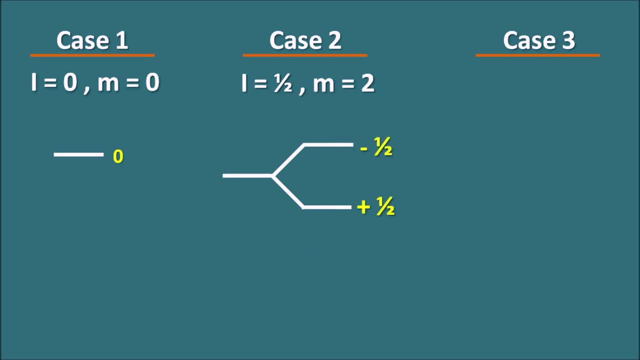 and another spin state is of the minus half. So plus half indicates the ground state and minus half indicates the exited state. Now in this case we can see that both of the spin states are equivalent, just differ in their sign. So these are having the similar magnitude but opposite signs. 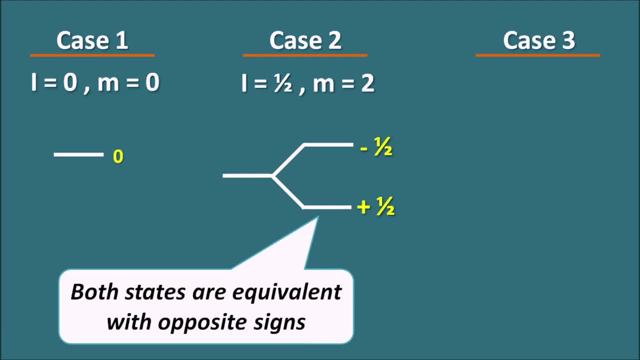 So such type of nuclei, These nuclei are perfectly suitable for the NMR spectroscopy. Now let us take the case three, where i is equal to one, then m is equal to three. Now nuclei can have three spin states: i is equal to plus one, i is equal to zero and 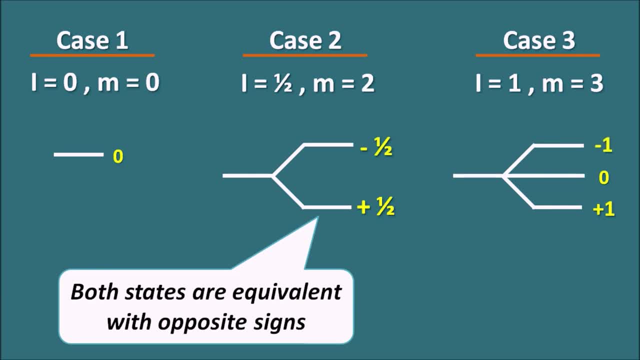 i is equal to minus one, And here we can observe that all these spin states are not equivalent. So we can see that plus one is having some spin, but zero is not having any spin. So these spin states are not equivalent, They are not suitable. 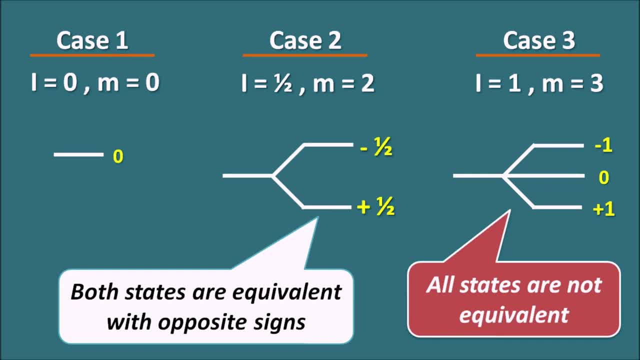 They are not suitable for the NMR spectroscopy. Here the distribution of the spin is not uniform, So we cannot observe a perfect NMR signal in the case three. So now the nuclei under the case one, where the i value is equal to zero, cannot give the.